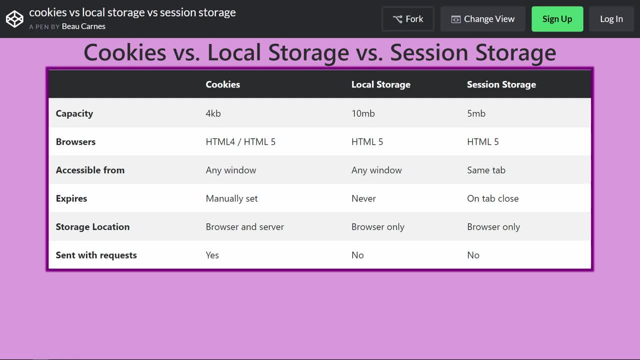 The capacity here is 4 kilobytes for most browsers, while local storage and session storage can hold 10 megabits and 5 megabits respectively. This means that cookies are going to be much smaller than local storage and session storage, but that's. 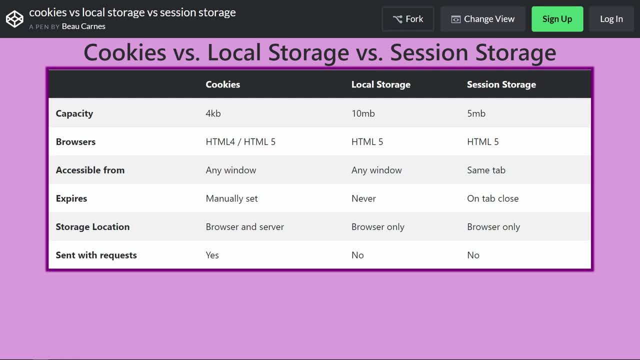 okay for their use cases. Also, cookies are supported in older browsers which support HTML4, because they've been around for much longer. but that's not really something you have to worry about because HTML5 is in pretty much any browser being used now. Also cookies. 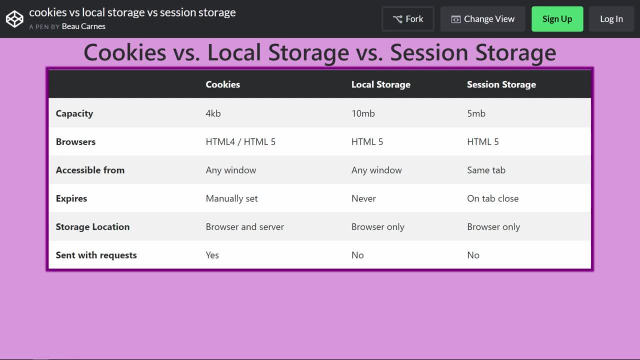 and local storage are available for any window inside the browser. so if you have Google Chrome open on one tab or another tab, the cookies are going to be available on all of the different tabs that you have open to that website, while, for example, session storage is only. 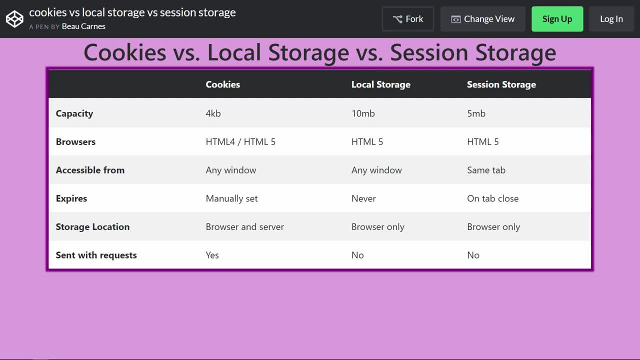 available in the single tab that you have open, that you set it in, so it won't be available if they open another tab and go to your website. As for expiration, this is where local storage and session storage really differ from each other. Session storage is for that one browsing session. 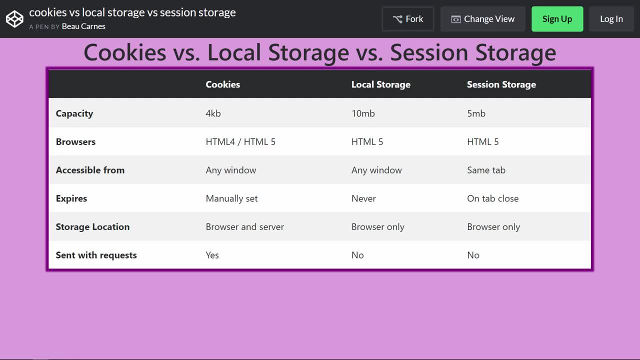 which is why it's called session storage, and it is removed as soon as the user closes the tab where that session was set, while local storage is around forever until the user ends up deleting it or you delete it yourself inside of the code, And then cookies. 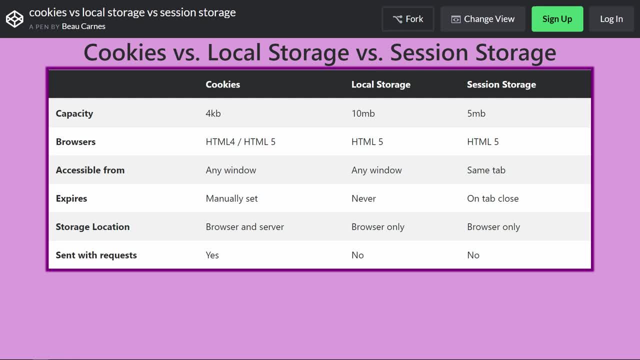 you actually have to set when they expire. Usually, you're going to either set an infinite expiration, for example, a year, very, very far in the future, or you're going to want it to expire in a certain time frame to see if the user has done something in that time. 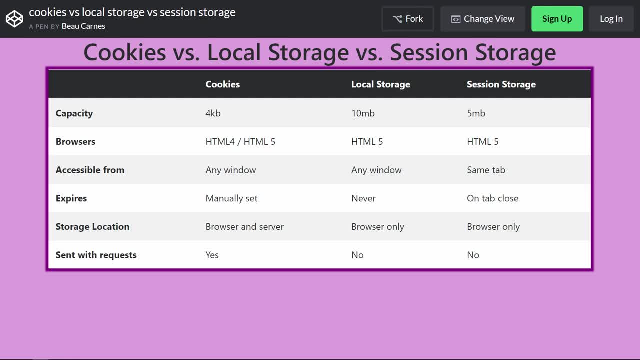 frame, but you have complete control over when the cookie actually expires. As for storage location, local storage and session storage are both on the browser, like I said earlier, but cookies, while they are stored in the browser, they are sent to the. 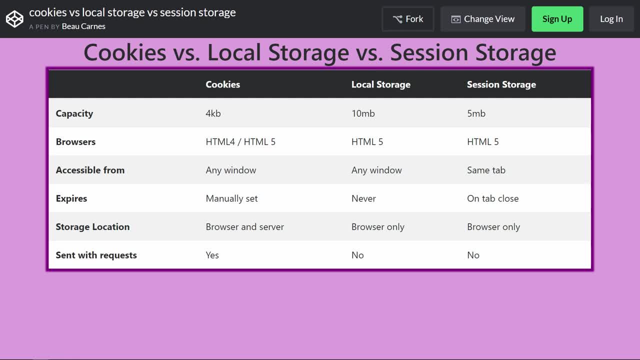 server. every time a user requests something from the server- whether it's an image, HTML5, file, CSS file, anything- the cookies get sent along with the request, which is why they have a much smaller capacity, because all of the information in the cookies gets. 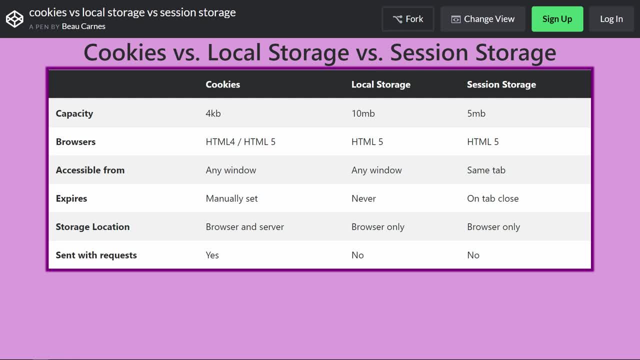 sent to the server. so if you have a lot of cookies that are really large, it'll slow down your request to the server and the request coming back from the server. This is why you want to make sure the cookies that you use are small and as limited as possible, so you 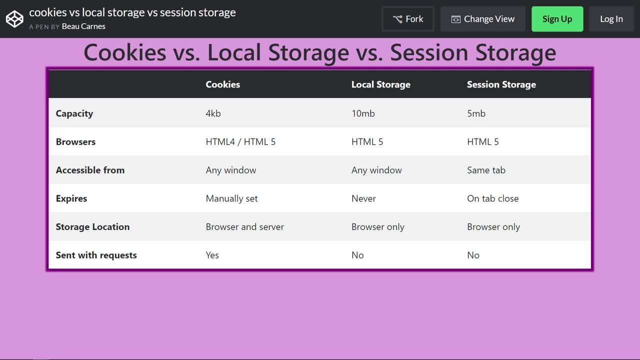 don't slow down the request any more than you need to. It also makes cookies really good for doing certain authentication-related tasks, because they actually get sent to the server every time a user requests something from the server. If you're going to be storing something in the user's browser, you're almost always. 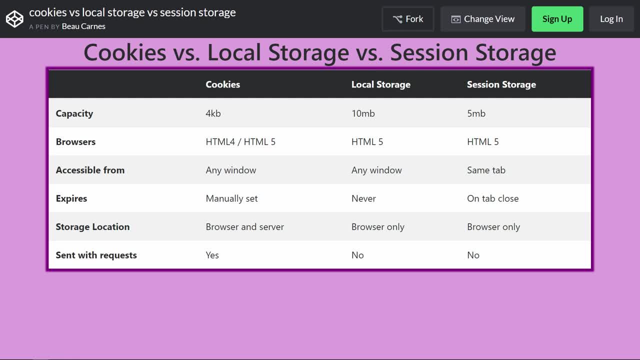 going to want to use local storage or session storage, depending on how long you want it to live, whether you want it to be for one session or if you want it to live after they close the browser and you only really want to use cookies if you need the aspect of sending. 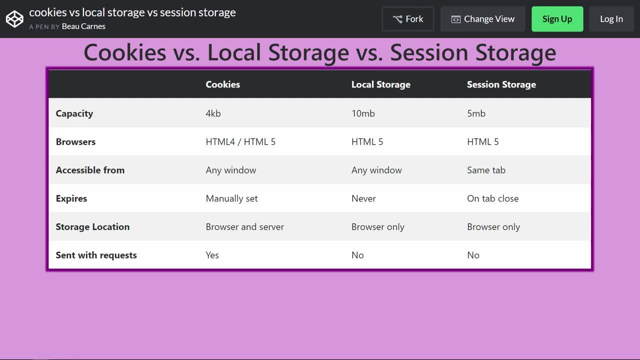 it to the server, because if you don't need to send it to a server, you're just going to be adding extra overhead, and cookies are much harder to deal with. so you should always use local storage or session storage unless you need to send it to the server. 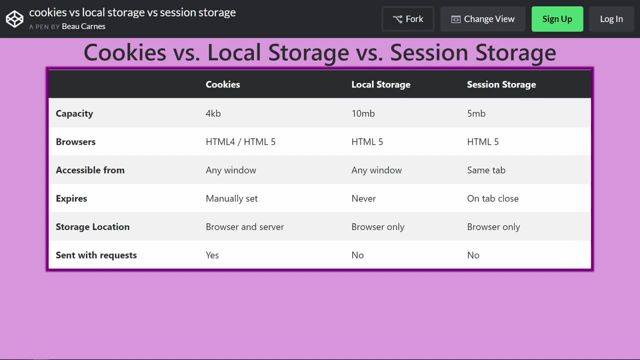 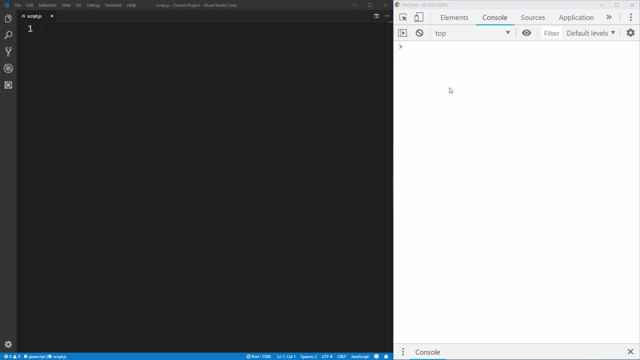 So now let's look at a few examples of cookies, local storage and session storage Over here. I have Visual Studio Code open on the left and I just have my Chrome Dev Tools open on the right for the webpage, so everything I type inside of my script is going. 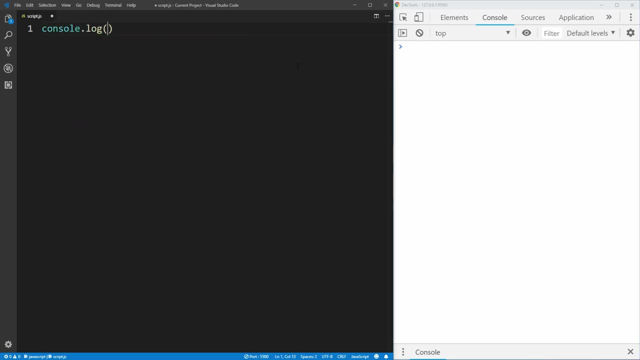 to show up in the console. here, For example, we could just do a log, we could just say hi, and if we save that, you see that's going to show up in our scripts over here. You can see our scripts over here on the log. 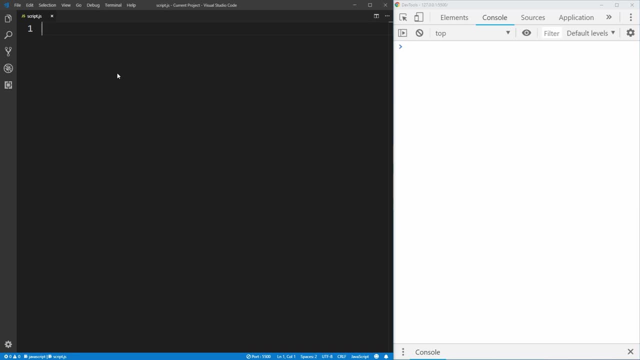 So if we wanted to start messing around with the actual different storage mechanisms of local storage, session storage and cookies, we need to figure out where we can view that information. in Google Chrome Dev Tools, And right here, this application section is where all that information is going to be stored. so if you click on that, you'll see we have. 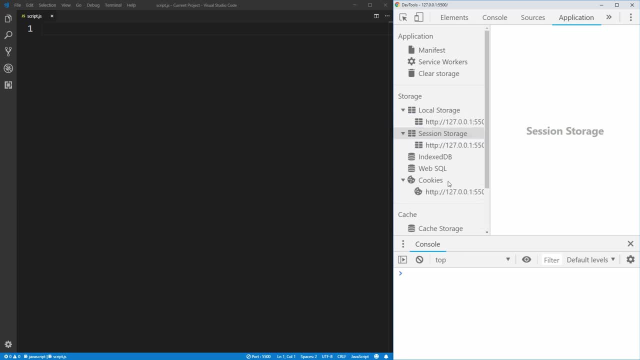 local storage information, session storage information and cookies available, and you can see that they're all going to be for this actual site that we're on, which is my local host. And if you don't actually see this up in the top, just click these little arrows on the. 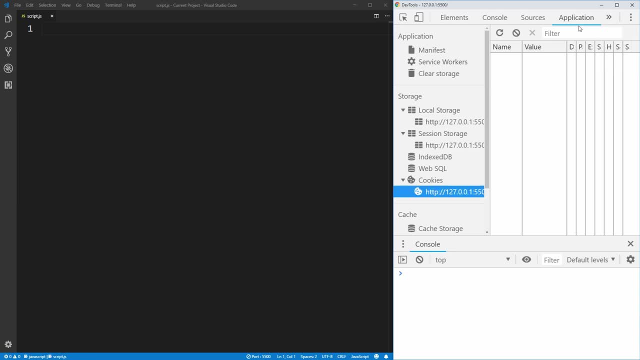 side and it'll be in the list over here for you, but for me it's just right on the top, so we can just go straight into it. You'll notice that at the beginning all of these are pretty much empty, except for my session storage. I'm using a plugin in Visual Studio. 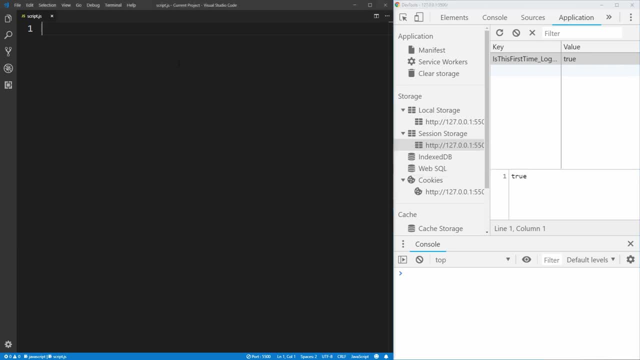 Code called Live Server. so every time I save my JavaScript it'll reload my browser and it just uses this session variable inside of that plugin. so we can ignore this variable right here for now. And then also my cookies are completely empty. 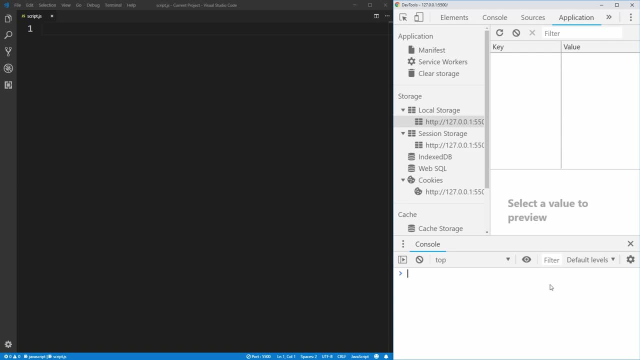 Let's start with creating some variables and adding them to our local storage. In order to do that, we need to access the local storage variable in JavaScript. Just type in local storage, and we have a few methods here that we can use. We have the get item, which will 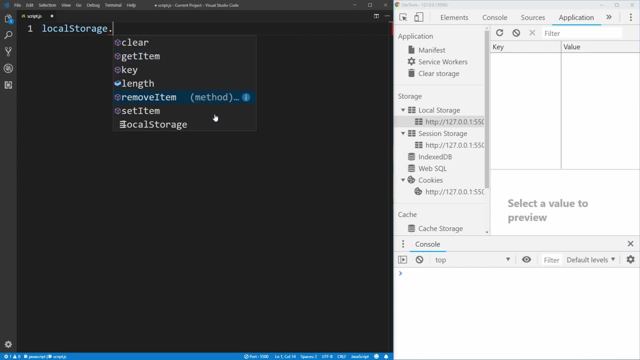 allow us to get something inside of the local storage, remove item, which will allow us to remove something. and then, finally, what we want, which is set item, which will allow us to set an item inside the local storage, And this just takes two parameters. The first, 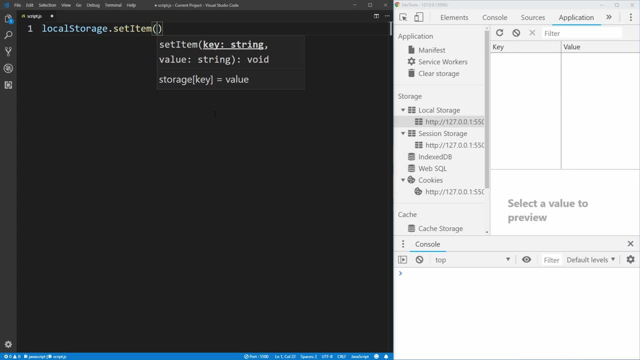 is going to be a key and the second will be the value. The key is what you're going to use when you want to get or remove something, and the value is what you're going to get when you get that keyed item. Think about this as a 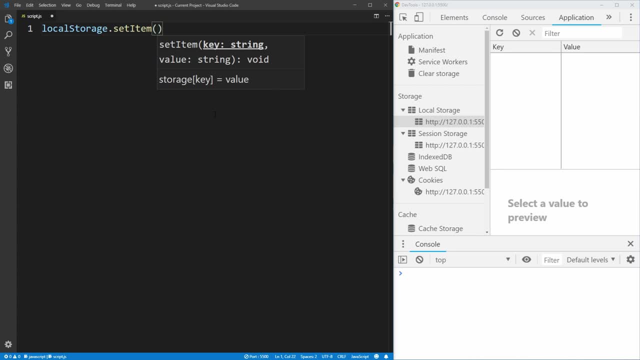 JavaScript object or a JSON object. You have your keys which are before the colon and then you have your values which are going to come after the colon, And in this case, everything has to be a string value and a string key. 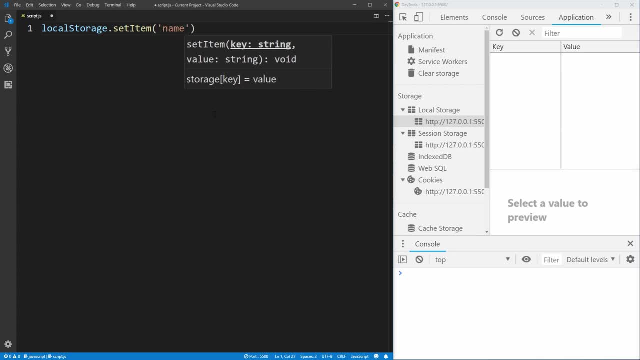 So, for example, if we wanted to put a name in here, we could put our name as the key and we could put the value of Bob, for example. And if you save that, you see that we now added this item to our local storage with the key name and the value of Bob And we 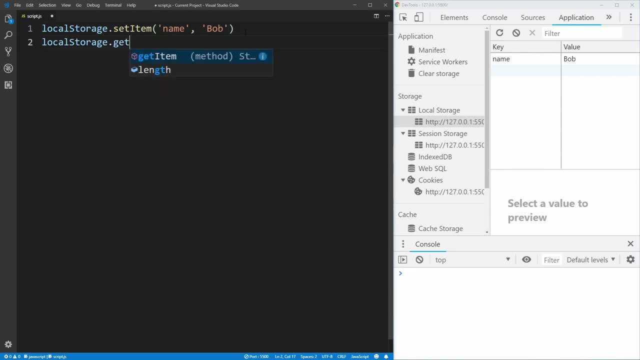 could get that item out of the local storage. so we could just say local storage dot get item and all we do is we pass the key that we added to the set item, which is name in our case. And to make sure this is working, we're just going to do a console dot log here. 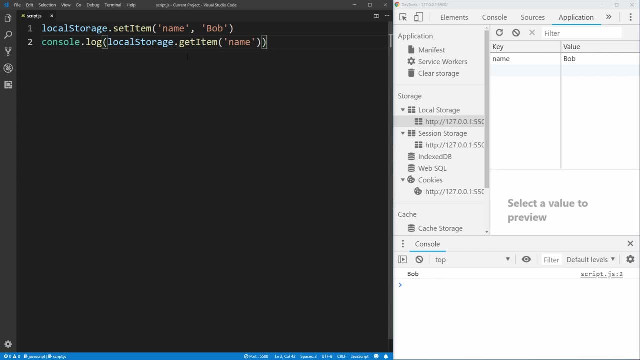 and if you save that, you'll see that Bob is going to show up in our log because it's getting that value from here in our local storage. And now, if we remove this line that we added and save it, you see that this local storage item is still in there, even. 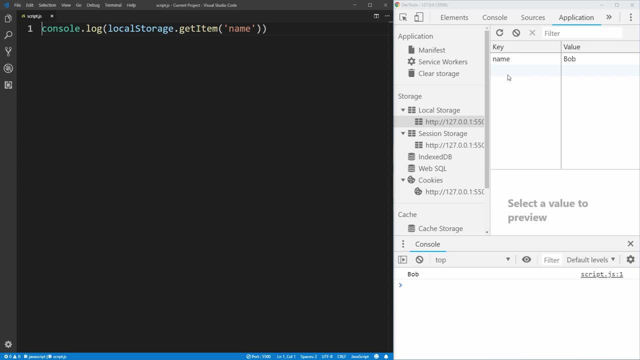 though we're not resetting it every time the page refreshes, And that's because local storage, like I said, is persistent, just like session storage, but session storage would end if we closed out of the browser. So now let me remove this, so we just click clear all, and now we no longer have that. 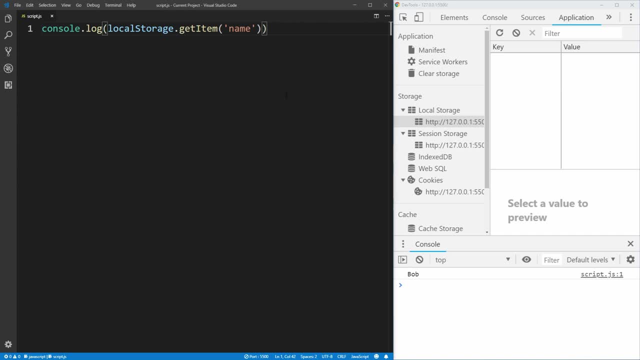 item in local storage. so we can see what happens if we try to get something that doesn't exist And, as you see, we just get null being returned, saying that it couldn't find the item that we're looking for. So let's go back here, add in the code to add that name back in there, so we have it. 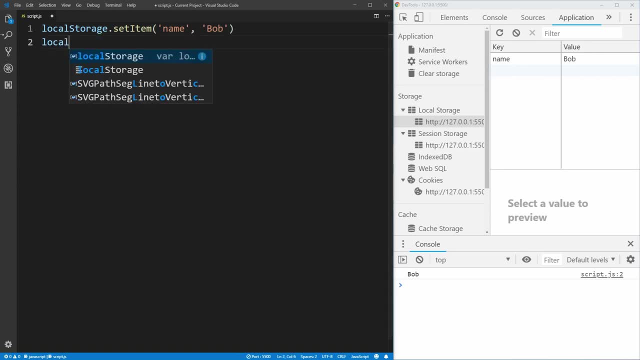 and then let's talk about how we can remove that item inside of the code. So we can just do local storage dot, remove item and again pass it the key we want to remove and if we save that, you see that that local storage item is completely removed. Now session storage. 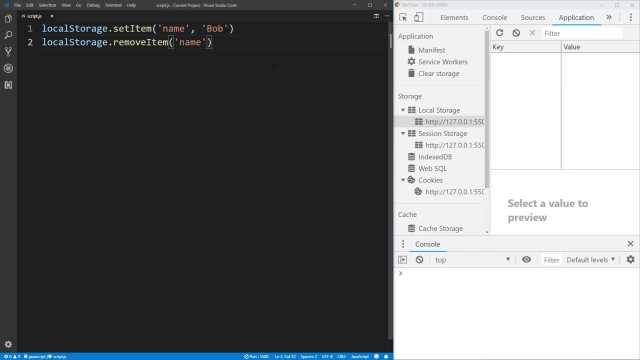 works exactly the same as local storage. All of the methods are exactly the same. so we just use the session storage object instead and, as you can see, we have our get item, remove item and set item methods And we're just going to quickly code something up here. We're going to do name again and 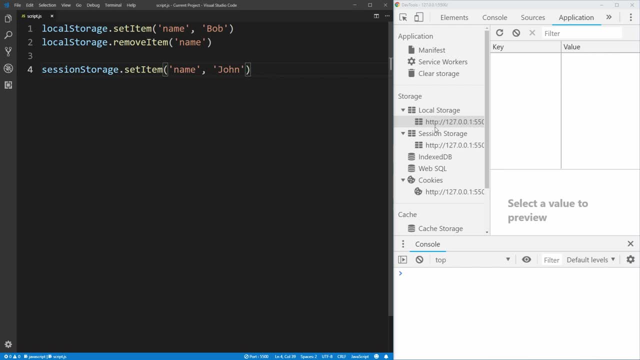 we'll just put John in here for this one and if we save that, go to our session storage section. you'll see we have name with the value of John. Then we can try to print that out, use that name key again. and we want to make sure that we actually log this and 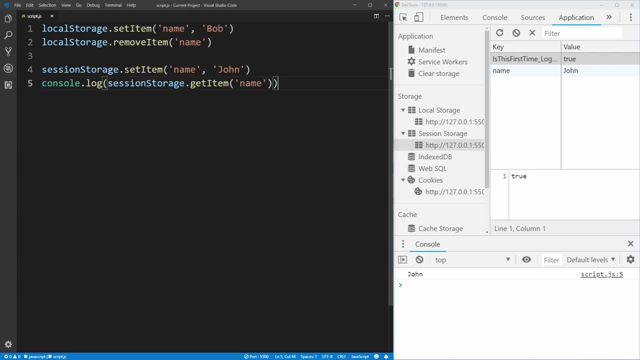 if we save that, you'll see that we're getting John printed out because it's getting that from our session storage. And then, lastly, we can do session storage dot remove item and we can again pass it the key that we want to get rid of. and if we save that, you'll see that our key is being 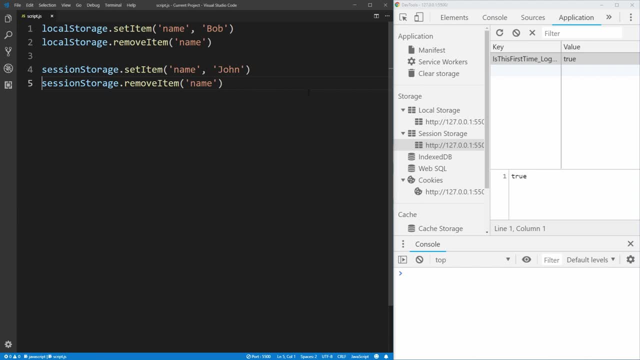 removed from the session storage and that's all there is to session storage and local storage. They're really straightforward to get working with and you can kind of think of them as like a JSON object or a JavaScript object, where you have key value pairs that you can. 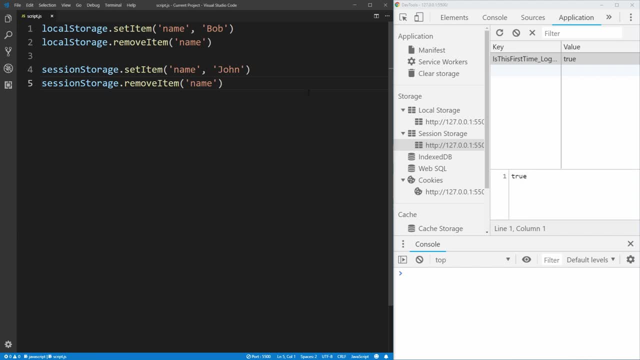 interact with by setting them and removing them. If you wanted to update something inside of the storage, If you wanted to update this name from John, all we would do is just do set item again, but we would just change what we want to set it to. so we can just set it to Bob and now. 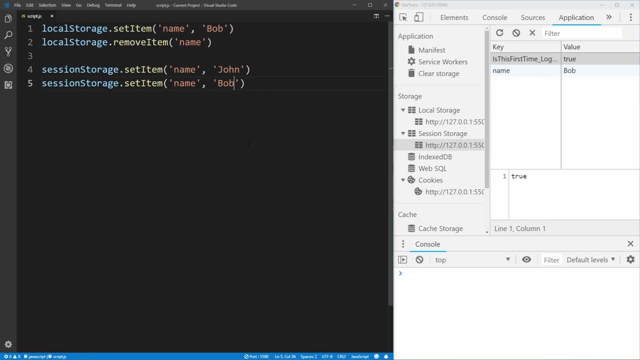 if we save that, you see, it overwrites the value to be Bob. Just like if you had a JavaScript object and you set a value of something that didn't exist, it would create it, and if you set the value of something that existed, it would just overwrite. 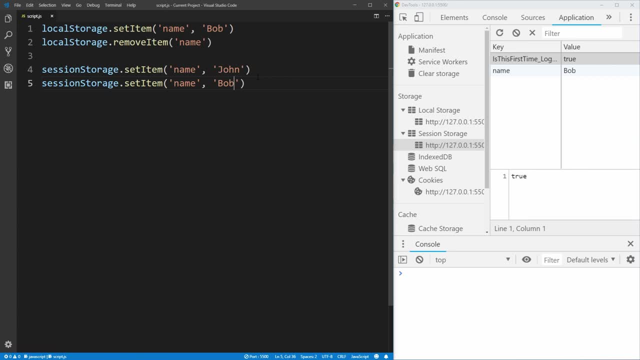 it. But then what we have left is cookies, and cookies are much more complicated and quite a bit different to work with than session storage and local storage, So let me explain how they work now. Unlike session storage and local storage, cookies don't have a very nice interface for. 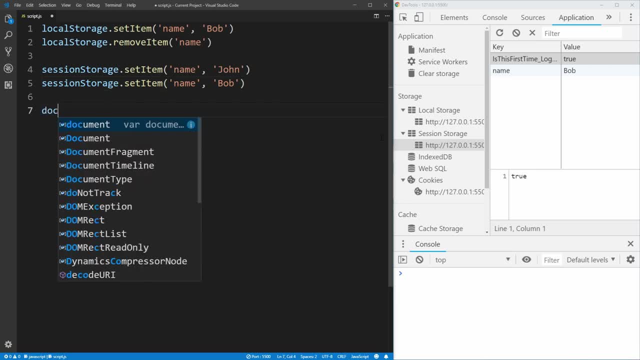 interacting with them. The only way we have to interact with cookies is through the documentcookie object and this object. both will allow us to see all the cookies and set new cookies. So if we wanted to create a new cookie, we would just set this value of cookie equal. 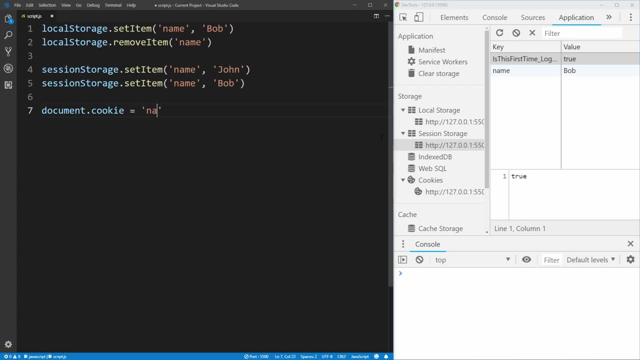 to the cookie we want to set. So in our case, let's say we want to set the name again and we're going to set it equal to another name. We'll just do Kyle, for example, And if we save that and go down to our cookies, you'll see that we have a name here, value. 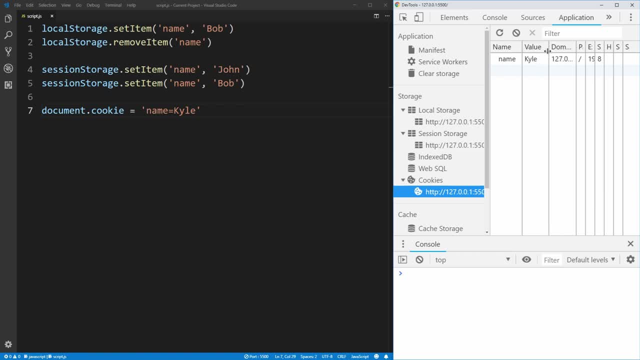 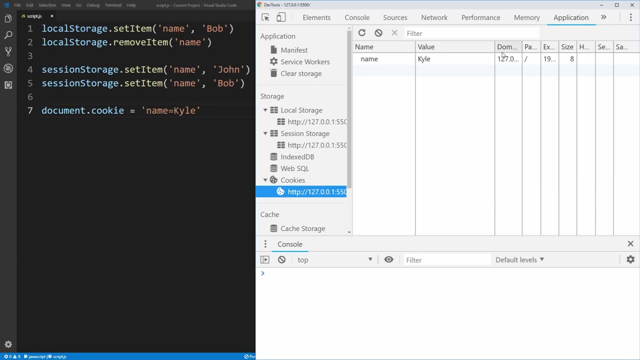 for name. We have the value of Kyle and then a bunch of other sections. here We have the domain that it comes from, the path that it comes from. Let me expand this so we can see it all easier. So we have the domain here, which is just our local host. 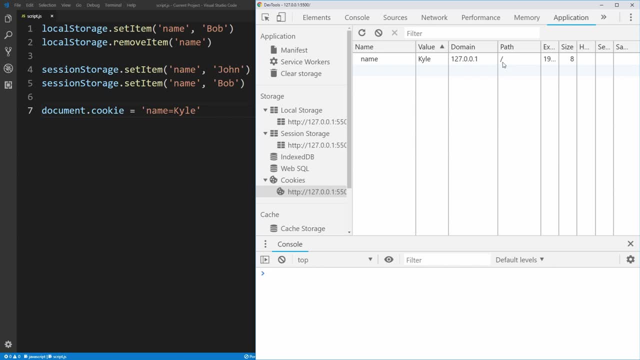 We have the path which we can set when we create the cookie. In our case, it just defaults to the page that we're on. We have the expiration and, as you can see, the expiration date is far in the past: It's 1969.. 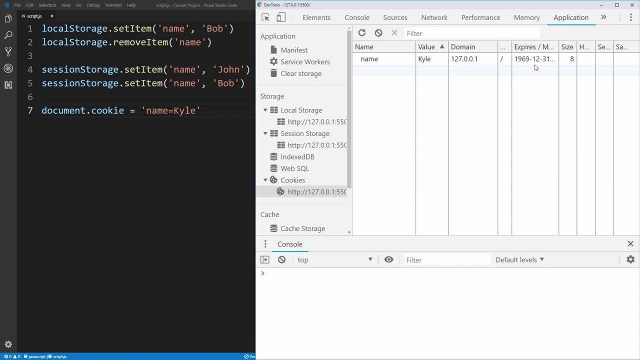 Because we didn't actually set a date that this should expire. so it's already expired. And then this is just the size. we don't really need to worry about that. So what if we wanted to set an expiration date for our cookie? 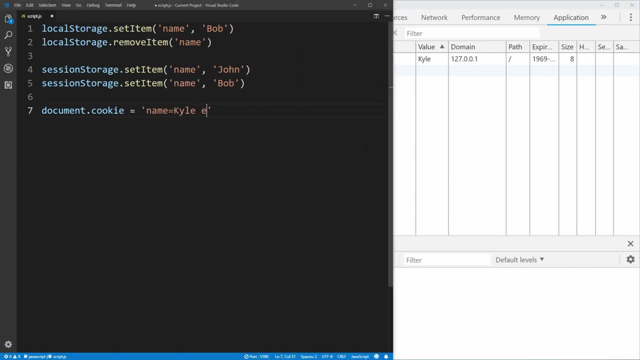 All we had to do is go into here and actually specify when we want it to expire. So we would put a semicolon here after our name to denote that we're going on to another section of our cookie, and then we just put expires and then we just want to put the. 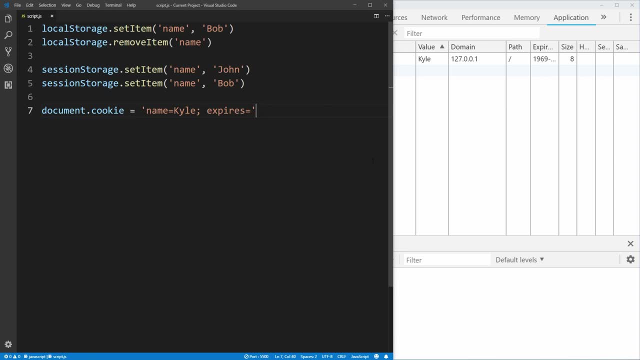 date that we want it to expire. In our case, we want this cookie to expire on January 4th, January 1st 2020.. So we need to add the UTC string of January 1st 2020 onto this expires token. 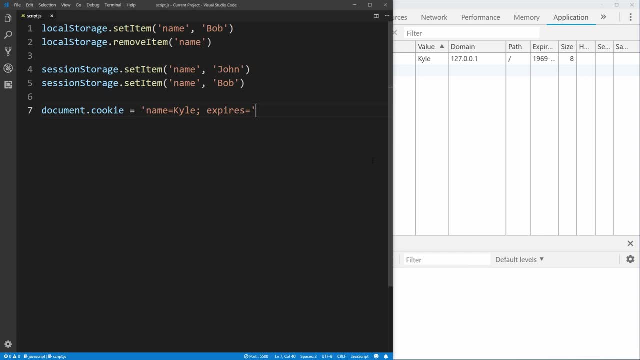 And the easiest way to do that is with JavaScript dates, because they have a toUTC string method on them, So all we need to do is create a new date. We want to pass it the year that we want 2020.. We want to pass it the date and the month, so the month will be zero here, because it's 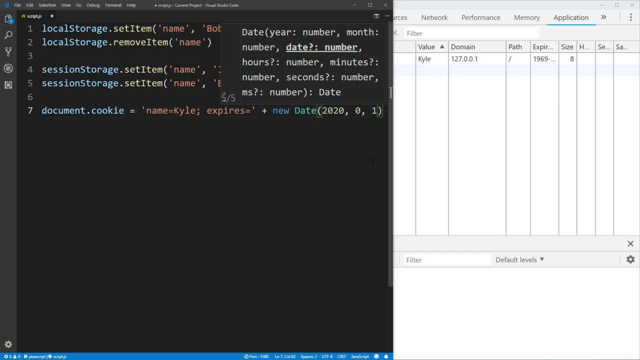 zero indexed and the date is going to be one. This is January 1st 2020.. And we can just save that. We just say to UTC string on this, and what this is going to do is it's going to append. 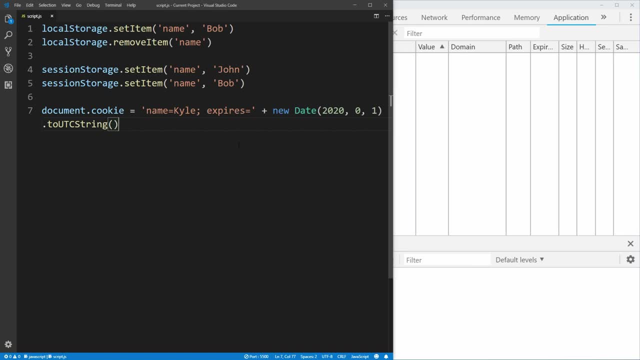 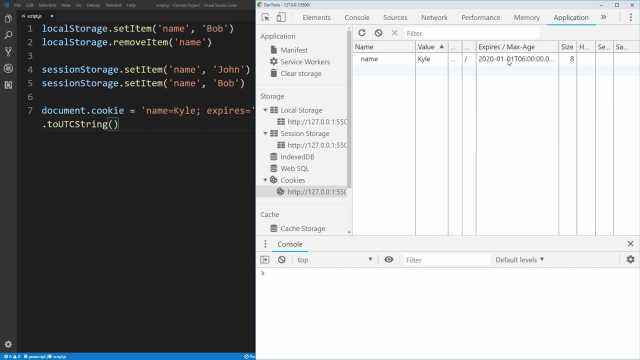 that UTC string onto our expires section. And now, if we save that, you'll see that our expire section here- if I can expand that, it expires on January 1st 2020, which is exactly what we want. If, for example, we wanted this token, our cookie- to never expire, all we would need 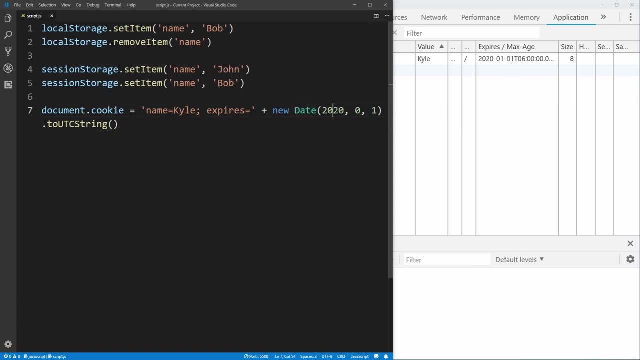 to do is just make a date that's so far in the future it'll never matter. So, for example, we can just put year 9999, and if we save that, you'll see that it now expires in year 9999, which essentially means it's going to never expire. 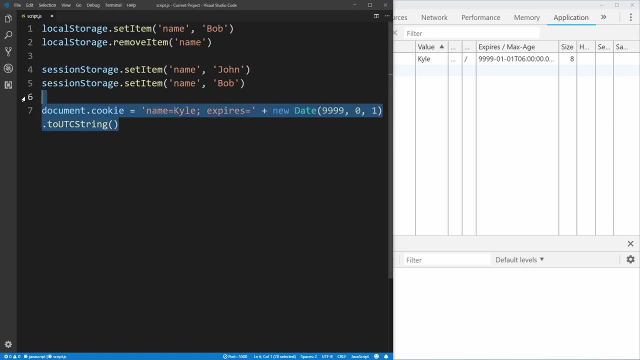 Now we can also add other cookies by doing this exact same thing. All we have to do is just say documentcookie equals and it'll add a new cookie instead of overwriting the old cookie. So let's just say we wanted to add another cookie. 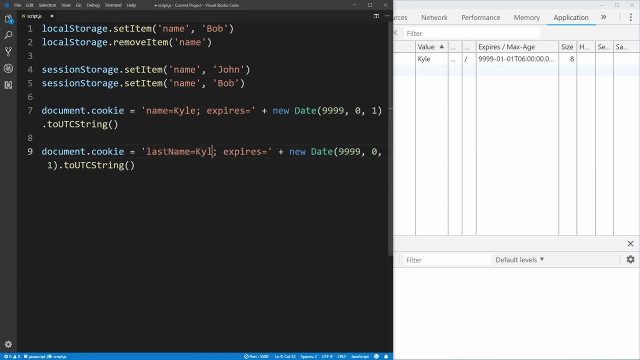 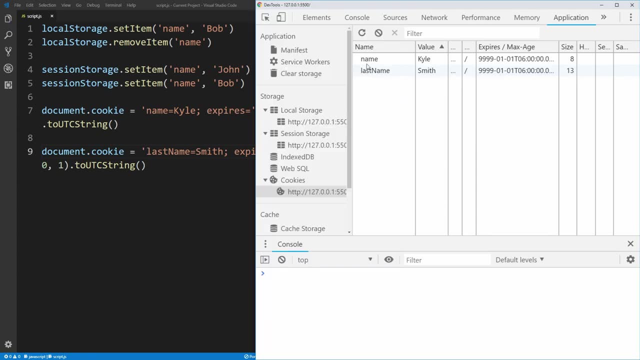 This time we're just going to say last name And here we can just set it to Smith And we'll also make it so it never expires. and if we save that, you'll see that we now have two cookies in here, even though it looks like we're actually overwriting the cookies. 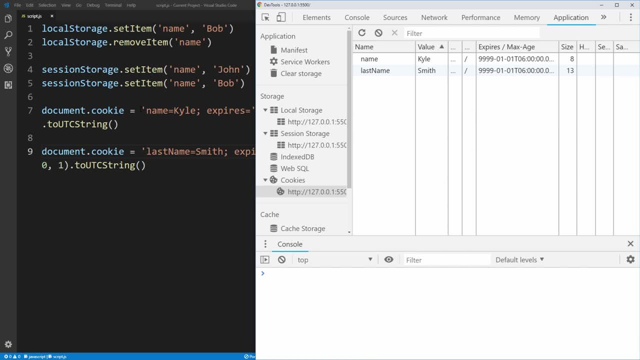 this is really just adding a cookie every time. we say cookie equals And if we want to view the cookies. there's no good way to view the cookies other than viewing all of the cookie information all at once. The only way we have to view them is through the documentcookie object. 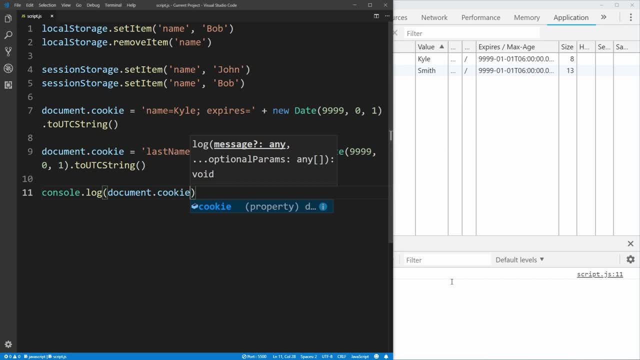 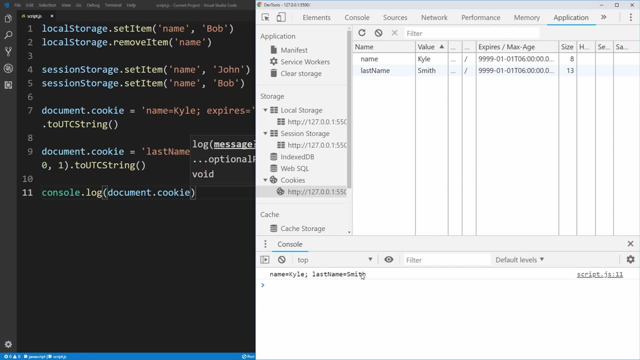 So we can just say documentcookie and if we print that out you'll see that it prints out: name equals kyle and last name equals smith. But there's no easy way for us to parse that other than just parsing the string itself. 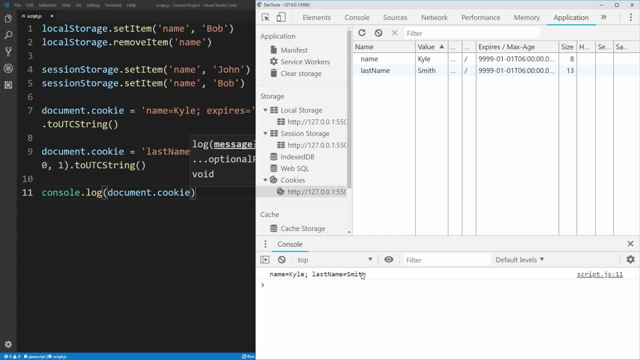 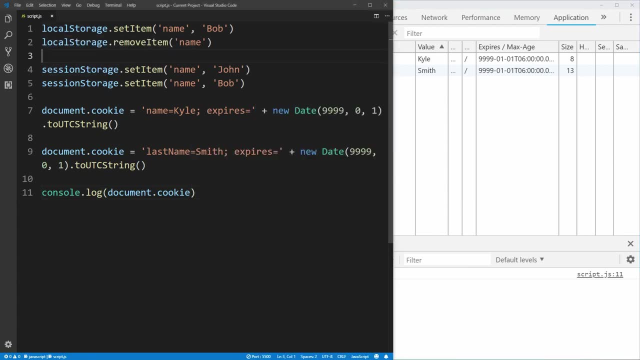 So I recommend, if you do need to work with cookies in any way, to use just a small library that helps manage cookies and makes them easier to use, kind of like local storage, and session storage are much easier to use rather than having to remember how to do all of this. string-related. 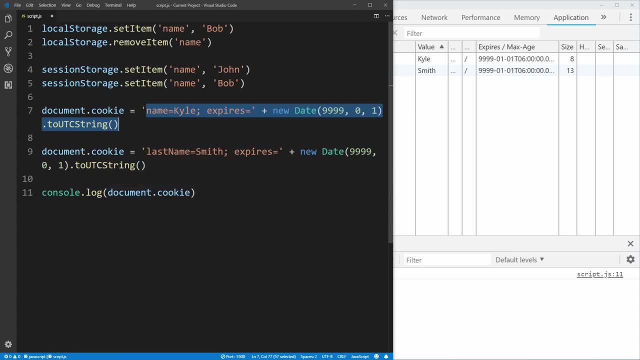 syntax and how to parse the actual documentcookie string that's returned. But, like I said at the beginning of this video, Most of the time you're just going to be using session storage and local storage, since those are stored in the browser and not actually sent to the server, and in most cases you